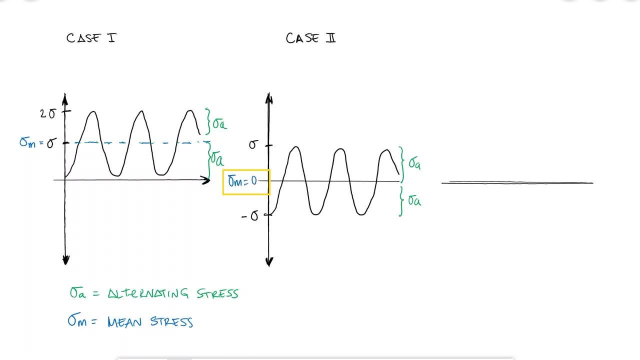 while case two's mean stress is negative sigma, Even though the alternating stress value is the same sigma. case two's mean stress is zero And case one is also not the same as a stress that goes from negative two sigma to positive two sigma, even though the maximum stress in both cases 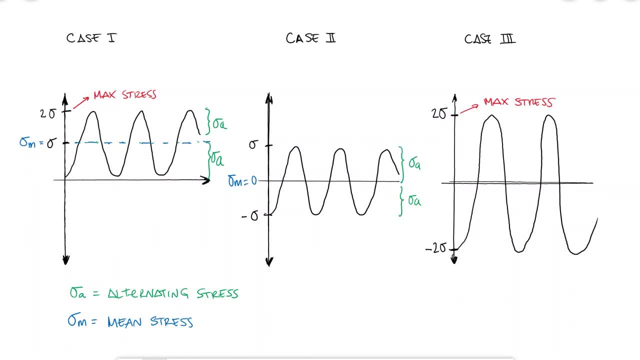 would be two sigma. We can say that case one is more taxing than case two because the overall maximum tensile stress in two never comes close to that of one. But case one is also not as taxing as case three because in case one we only have a maximum stress and tension of two sigma. 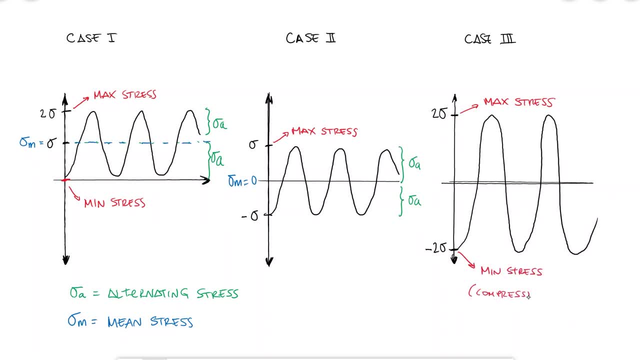 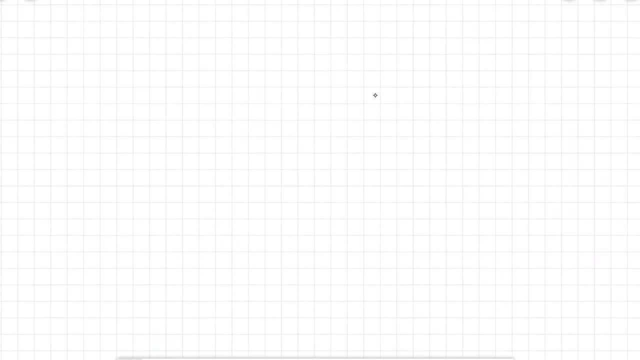 while in case three we have both tension and compression of two sigma. Let's think about steels for a minute and let's recall that the endurance limit is defined for one million cycles and above. If I have a plot for alternating stress on the y-axis and mean stress. 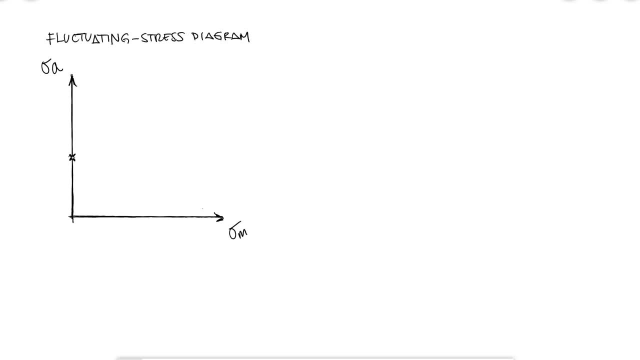 on the x-axis. from everything we've covered so far, I know that for a completely reversed stress, which has a mean stress of zero and an alternating stress of sigma a- meaning x equal to zero and y equal to sigma a- the part would fail when the alternating stress value is just above the 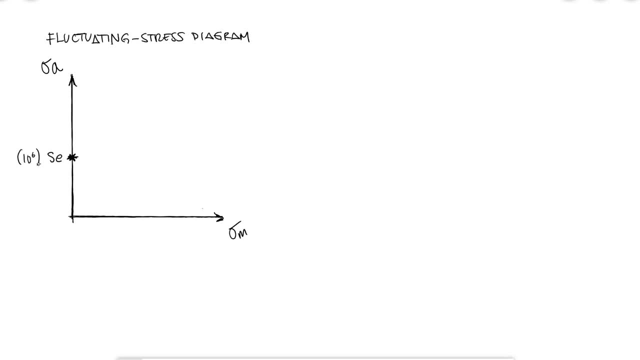 endurance limit. Of course, this is not the case for case two and case three, because they are not the same. The part would be required to be subjected to a higher stress if the number of cycles was reduced For 10 to the 5th cycles, the alternating stress can be higher and equal. 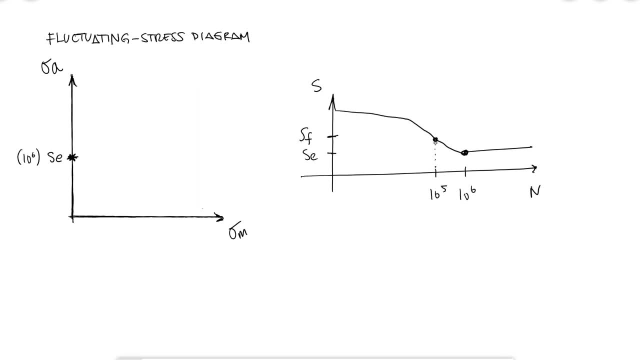 to the fatigue strength for 10 to the 5th cycles, for it to fail exactly at 10 to the 5th cycles, and so on and so forth, Regardless of the number of cycles, if the alternating stress is zero, which means the stress is just constant and equal to sigma m and therefore it does not fluctuate. 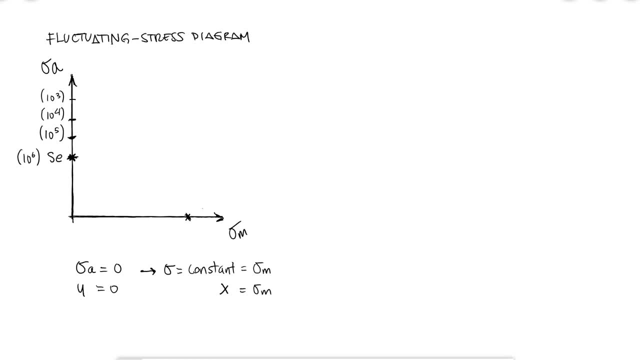 I know the part will fracture when sigma m is equal to or exceeds the ultimate strength. These are called the constant life curves on the fluctuating stress diagram. There are situations where you know a part will only operate for a known number of cycles, situations for which you will want to calculate the factor of safety. 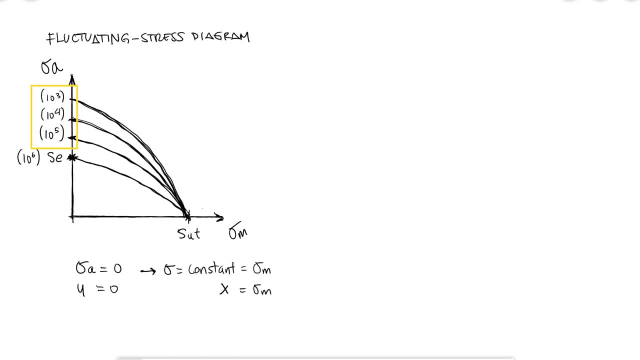 and therefore the fatigue strength for a specific number of cycles, like we've been doing in previous videos. But for many, many applications, you just want to design a part to have an infinite life. So we'll focus on endurance limits for now and up to this point. 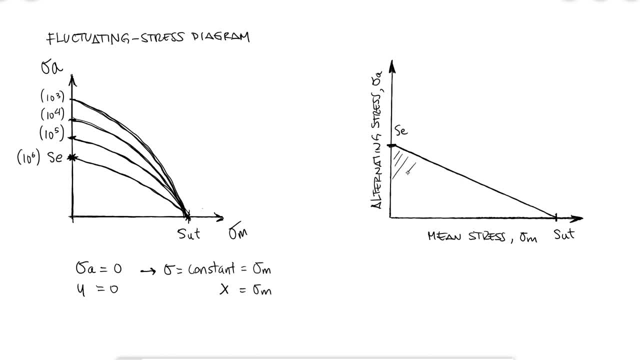 we would assume that any combination of sigma a and sigma m within this triangle would not cause the part to fail. The factor of safety would be calculated, just like we did with static loading, as the ratio between the length of the line from the origin to the safe line. 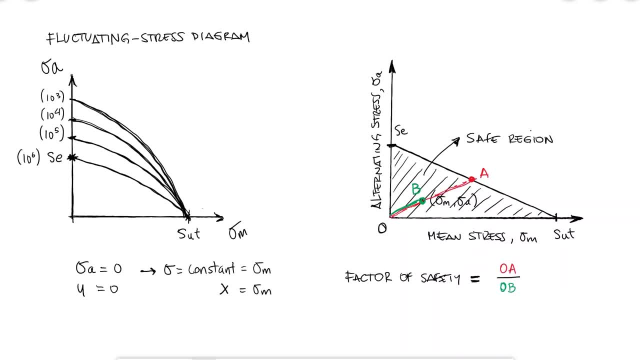 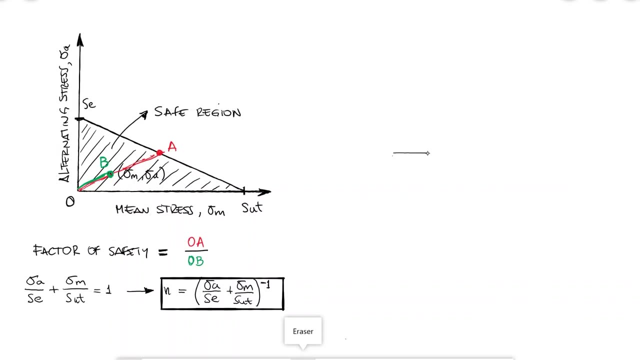 and the length of the line from the origin to the stress state, which follows the same expression that we derived when looking at the failure criteria for static loading. Since, for many applications, exceeding the yield strength is considered failure as it would cause plastic deformation, we add an extra boundary line for the combination of sigma. 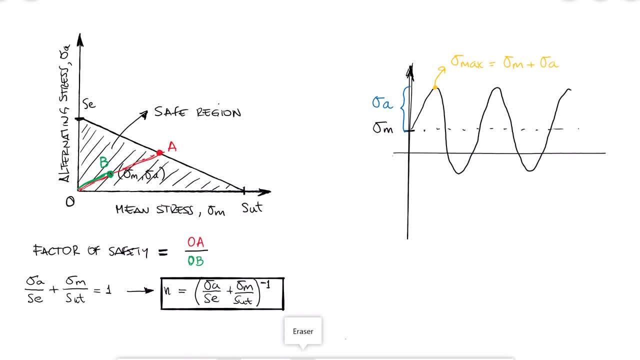 a and sigma m that, when added together, which will happen at some point during the stress cycle, would exceed the yield strength which happens whenever a stress state is located above a line bounded by Sy in the y and x axes. This would, of course, change what I just explained on how. 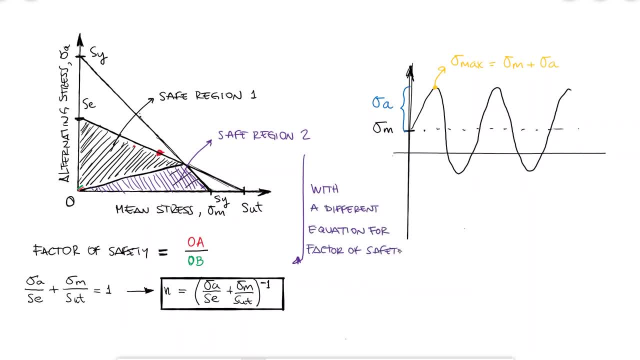 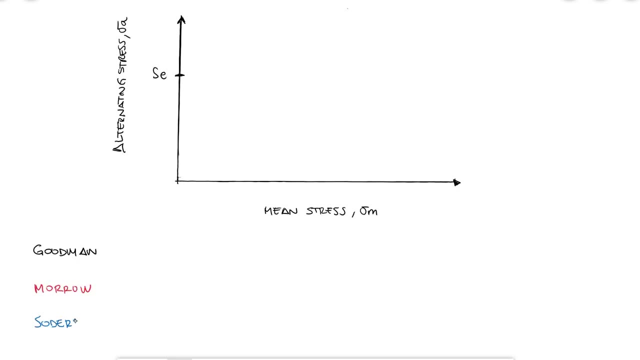 to calculate the factor of safety, creating two different regions. Fortunately for us, the fatigue failure criteria curves that follow what experimental data yields are already functions that more easily mathematically define the factor of safety. We have straight lines for Goodman Morrow and Soderbergh, where Soderbergh uses the yield. 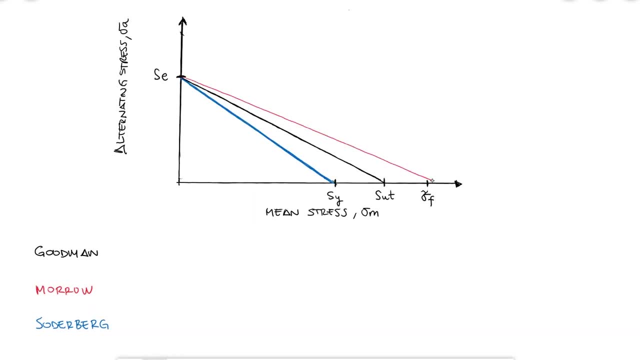 strength. Goodman uses the ultimate strength and Morrow uses the true fracture strength. Remember that true fracture strength that I talked about several videos ago. This is where we use that, But these are too conservative. Lab results we already know show that curved or elliptic plots fit the data better. 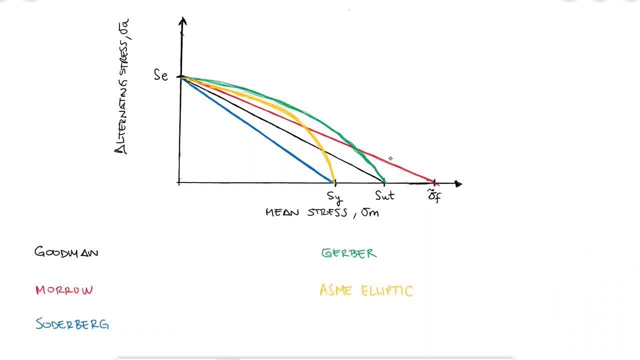 like the Gerber or the ASME elliptic criteria. One criterion that does not simply attempt to fit experimental data is the Smith-Watson-Topper criterion. It uses theoretical bases and strain life methods to delineate the boundary. and since it doesn't converge to zero, 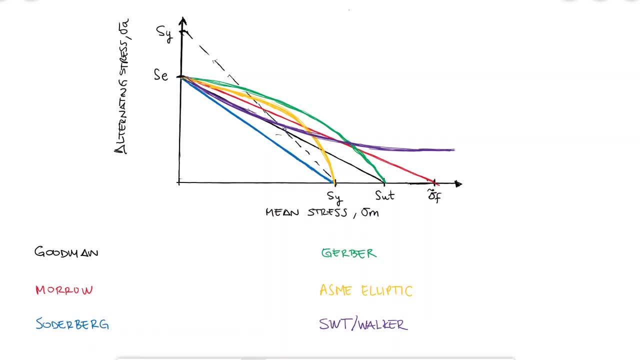 it's usually used in combination with the yield strength to yield strength line we discussed before. Mathematically, there will be a design equation for each one of the criteria. We already know what the straight lines look like with, once again, Goodman using the ultimate strength. 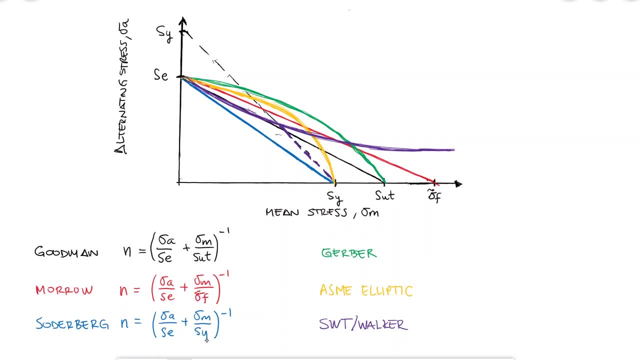 Morrow using the true fracture strength and Soderbergh using the yield strength For Gerber and ASME elliptic. the definitions are pretty easy, where you have a squared term for the mean stresses in Gerber and each one of the two terms squared for the ASME criterion. 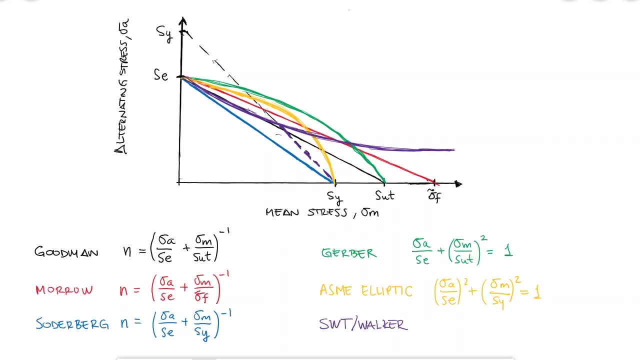 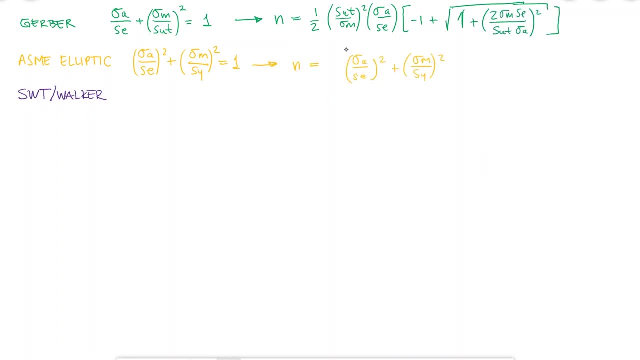 By using these function definitions and carrying out a similar procedure to the one I explained before for calculating the factor of safety, we obtain the expressions for factor of safety for each one of the criteria. Let's take a look at a quick example now. 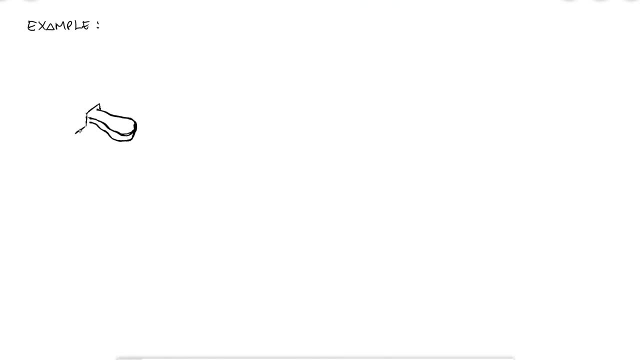 The pedal of a piano is a part that is pressed on many, many times during its lifetime. As you press down, the pedal swings around a hinge that initiates the movement of the rest of the mechanism. When the motion stops but the load is still there, the pedal is effectively. 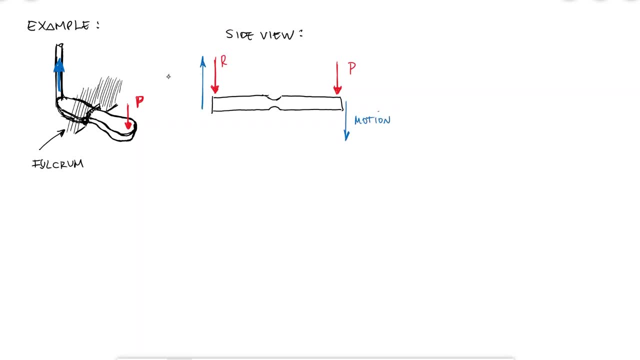 subjected to bending, Even though the motion of the opposite side is in the upward direction. the reaction force is going downward And if we were to look at the cross-section of the pedal we would see that it's not a solid rectangle. Of course we can do all the calculations to find. 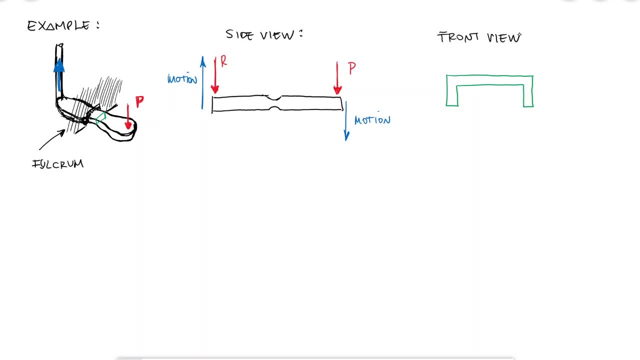 the second moment of area, for example. But for the purposes of this example, which focuses on fatigue failure criteria, we will simplify it as a rectangle of 1 by 1 fourth of an inch, And I know that the radius of the notch around the hinge is equal to 1 over 32 inches. 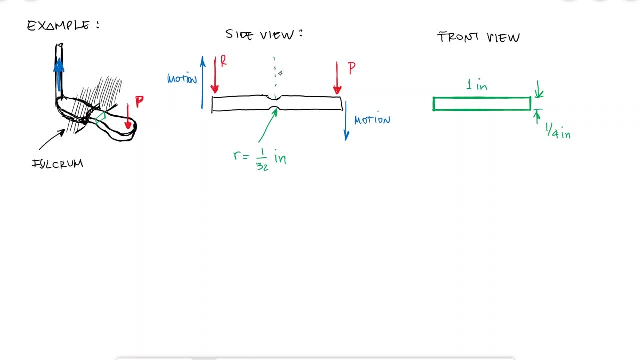 Assuming the pianist puts a lot of their weight on the pedal when playing intensely, we will assume a load of 40 pounds. I would like to estimate the fatigue factor of safety based on achieving infinite life using, for example, the Goodman and the Gerber. 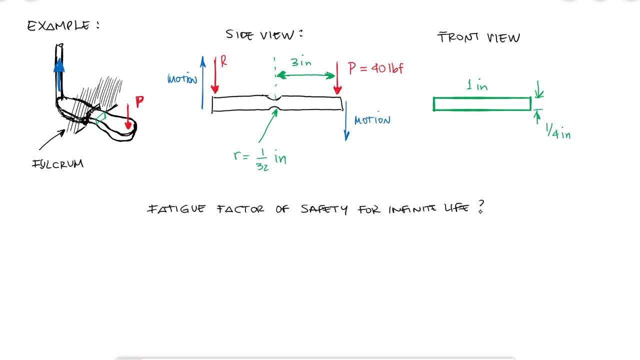 criteria. Remember once again that all of these problems have two independent processes. The first one has to do with the strength, or, in general, the material properties, and the second one has to do with the stresses. Let's begin with the strength, or, in this case, the endurance limit. 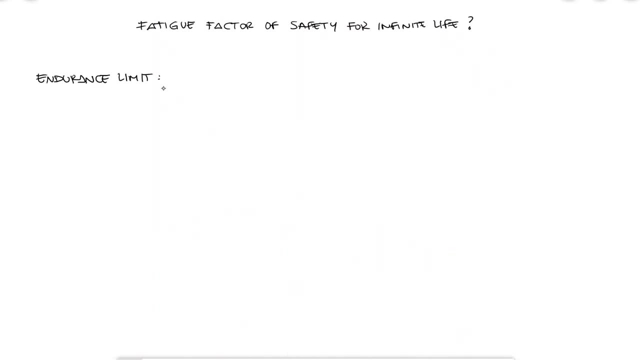 since I'm interested in the infinite life. A piano pedal is probably made out of brass, but let's assume it's just a steel, so that we can use the plots and equations that we've grown familiar to. The ultimate strength of the steel I'm using is equal to 77.5. 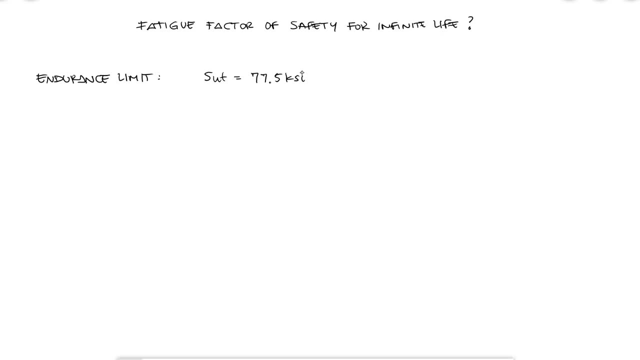 ksi. Since I'm not trying to find a fatigue strength and therefore I don't need the SN diagram, I won't be needing to find the F coefficient for the F times SUT term. I just need a first estimate of the endurance limit SE and a more accurate one using the marine factors. 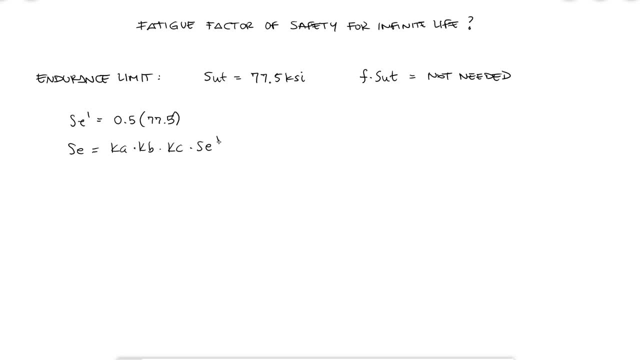 As with a real brass pedal, the surface finish would probably be a polished one and therefore the surface factor would be equal to 1.. Using the equivalent diameter equation for a rectangular cross section, I would find that the equivalent diameter is 0.404 inches. If I use that value, which is between 0.3. 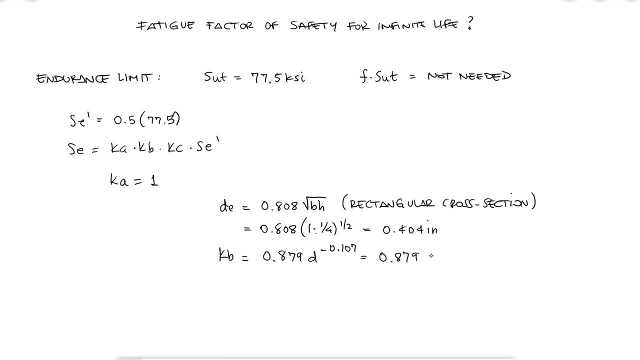 and 2 inches to calculate the size factor Kb, I would find a value of 0.969 for it. Since the loading the pedal is subjected to is bending, Kc would be equal to 1.. And since the temperature will probably just be the room temperature and my calculations are looking 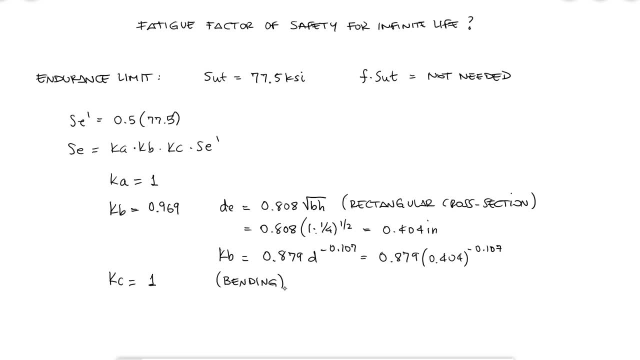 for a factor of safety. I'm going to calculate the size factor of Kb And therefore I don't need the reliability factor. Kd and Ke would be equal to 1 as well. But that's it. A better estimate for the endurance. 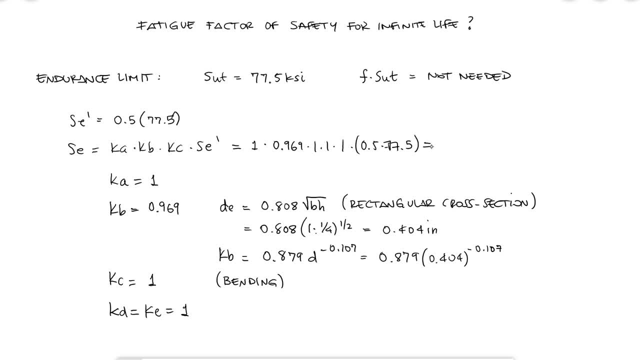 limit using the marine factors yields a value of 37.5 ksi, And this is half of what the problem was asking for, since I now have the endurance limit and the ultimate strength, the two properties that I will need for my factor of safety calculations. 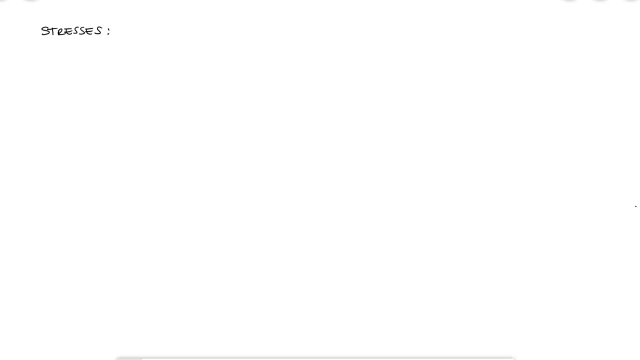 The second step is regarding the stresses, And here I'm trying to identify the values for the alternating stress and the mean stress, And this is mostly mechanics of materials with a little bit of fatigue. when trying to find the fatigue stress concentration factor, I know that the maximum stress is equal. 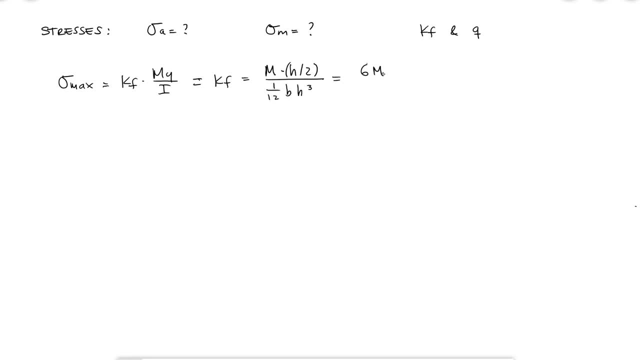 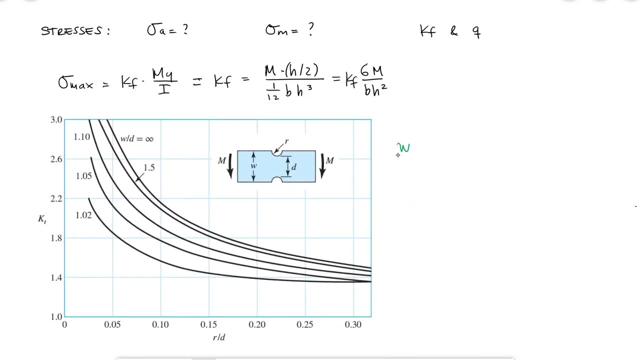 to the stress concentration factor for fatigue times MY over I. For a notched rectangular bar in bending like this one, I will need the W over D ratio and the R over D ratio, Where W is 1, 4th of an inch, the notch radius 1 over 32 of an inch and therefore D 3, 16ths of an inch, which result in: 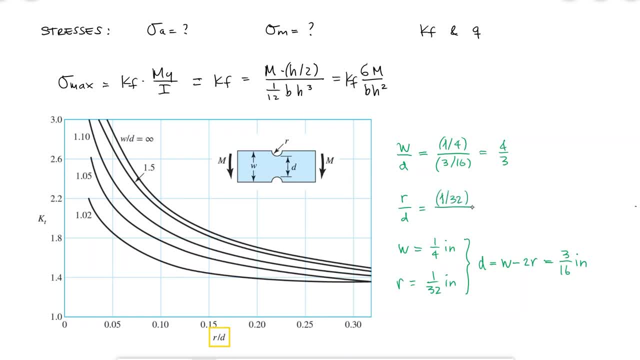 ratios of 4 3rds and 1, 6th or 0.16 repeating. Looking at the value for the static stress concentration factor kT, I would find a value of 1.7.. And if I look for the notch sensitivity value, 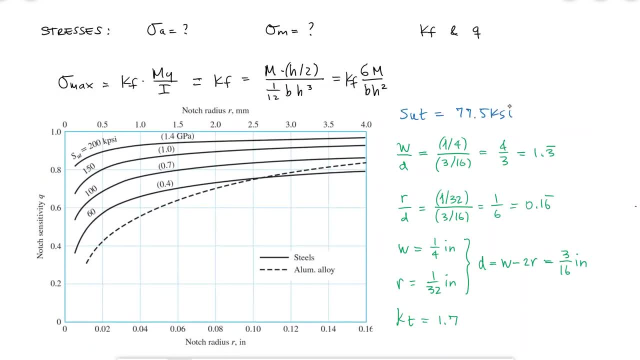 for a material with an ultimate strength of 77.5 ksi and a notch radius of 1 over 32 of an inch, I would find a notch value of 1.7.. Using these values and the expression we obtained during the last video, we find a fatigue strength.